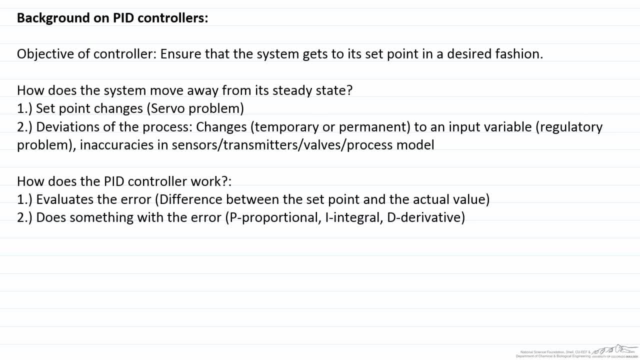 temporary, just momentarily. they can last for a few minutes, or they can be a permanent change due to some modification of the process. These changes can happen to some sort of input variable. It could be the manipulated variable, the variable which has the valve or pump on. 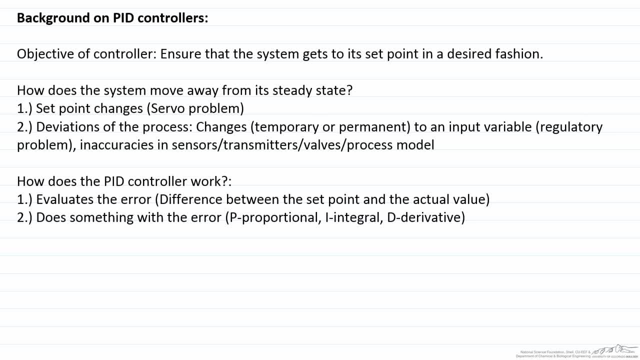 it which is doing the controlling action of this process, or it could be some disturbance to the process which is not being measured or controlled. Either way again, take me the example of temperature inside a reactor. any of these things can cause the temperature. 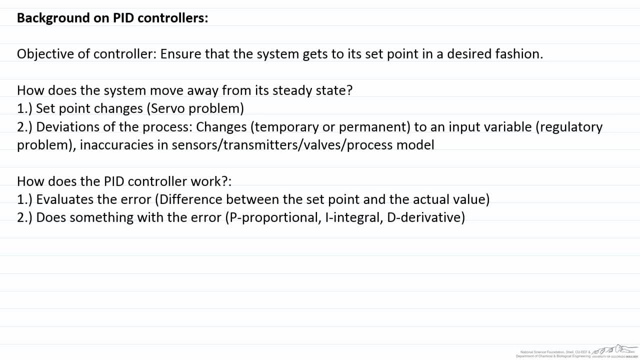 inside the reactor to change. Additionally, there could be inaccuracies present in sensors, transmitters or valves which could cause small fluctuations. but again, these fluctuations still do occur and our controller needs to be able to handle that. So what the controller does is it does two things. The PID control the first thing. it 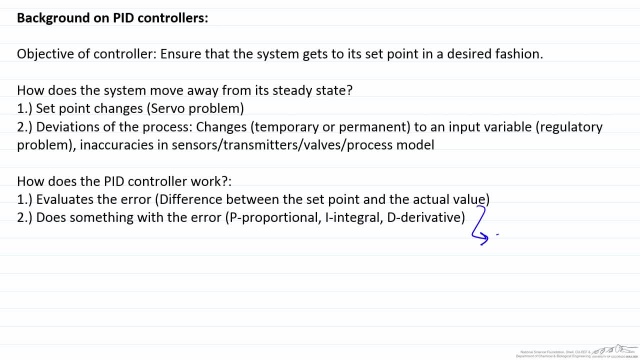 does, is it determines the error. so therefore, in a controller, the error is defined as the difference between the setpoint value and the measured value, And the way this has been assigned is solely more from a convention standpoint. So once it calculates this error, 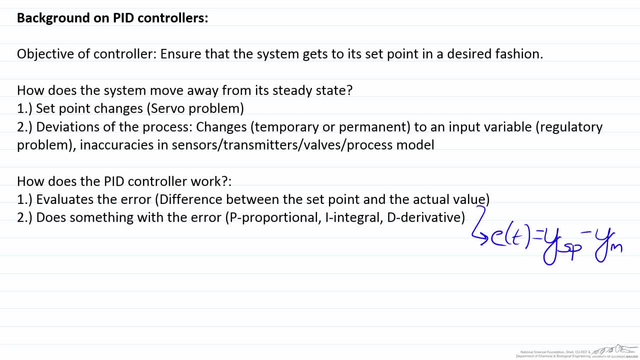 again. typically this error is calculated in some sort of electrical signal: percent, controller, output, milliamps, etc. Once it calculates the error in some terms of signal, what the controller then does is it can take the proportion of the error, it can take the integral of. 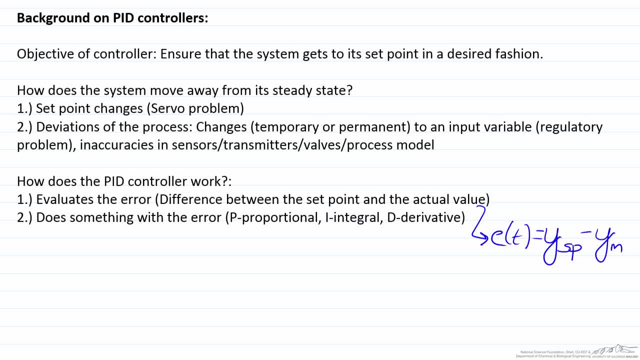 the error, or it can take the derivative of the error. Depending on the type of controller, it can do one, two or all three of these things. So we will now take a look at how each of these controllers- PI and D- work together and work individually. So we will first start. 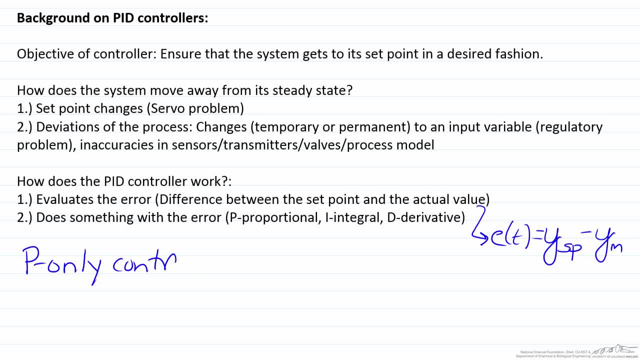 with proportional control by itself, which is often known as P-only control. And what P-only control does is it takes the error and it finds a proportion of it where this proportion is represented by Kc, which is the controller gain. So the equation that 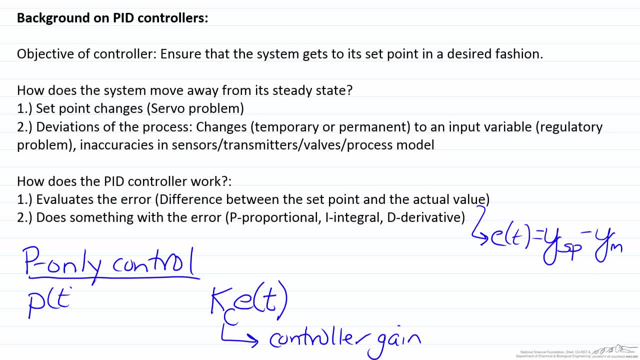 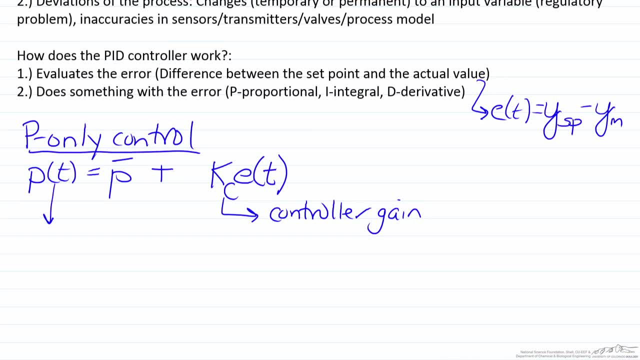 represents P-only control is represented as: P of t equals P bar, plus this Kc times P times E. So P represents the actual value of the controller output and P bar represents the bias. The bias is another way of saying at what percent controller output or at what. 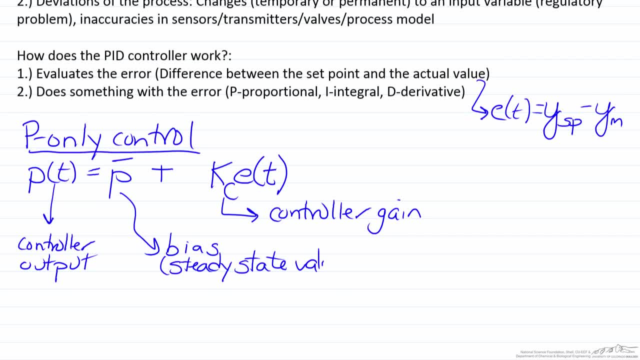 milliamp signal should this process be, if everything is okay and there is no error and it is at its steady state. So often times this is set to 50% controller output, but be aware that this is not a necessity, Sometimes depending on how the controller output is. 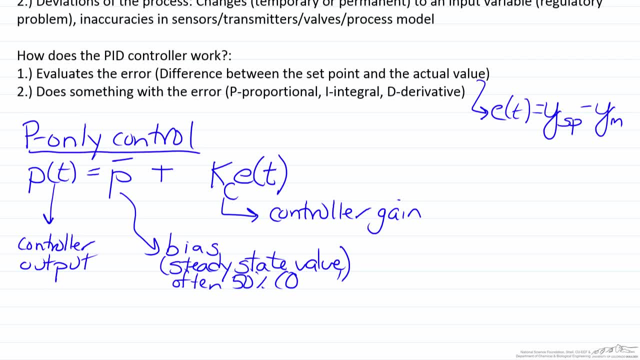 how the control systems connect together. this value could be something different. An important point to note here is that the controller gain must be the right sign, otherwise your process is going to be controlled in the opposite direction, making your process worse and worse. 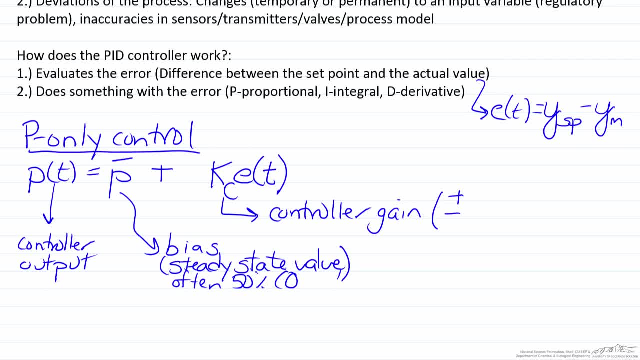 So by convention, partially based on the definition of error, plus here is defined as a reverse acting controller and minus is represented by a direct acting controller. There are techniques that can be used to determine whether or not your controller should be reversed. This is the representation of P-only control in the time domain, In the Laplace domain. 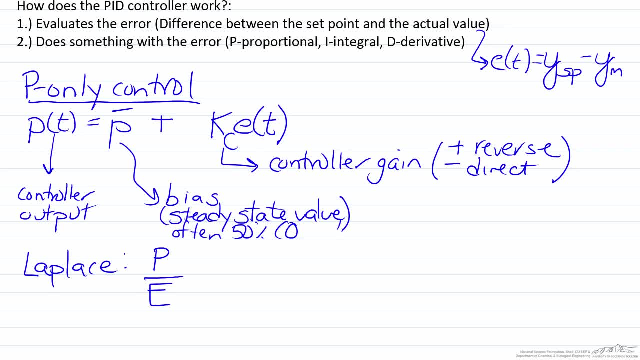 it is simply P over E, where the P here is the controller output, again in the Laplace domain, and E is the error in the Laplace domain. This is simply a zeroth order function, K sub C. So a major advantage of P-only control is the fact that it is fast responding, which? 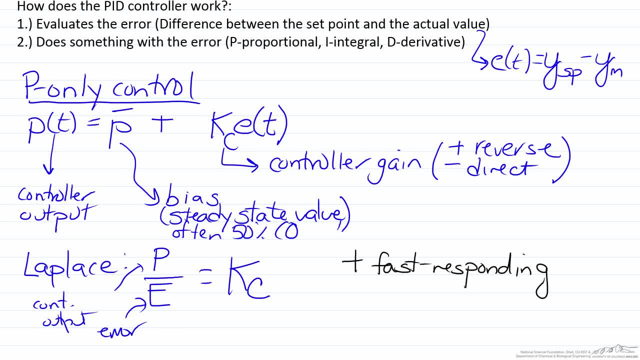 can be seen by the fact that it is a zeroth order transfer function. But the major issue that we have with P-only controllers is that there is always an offset. In other words, the process will never reach the desired steady state, and this term is. 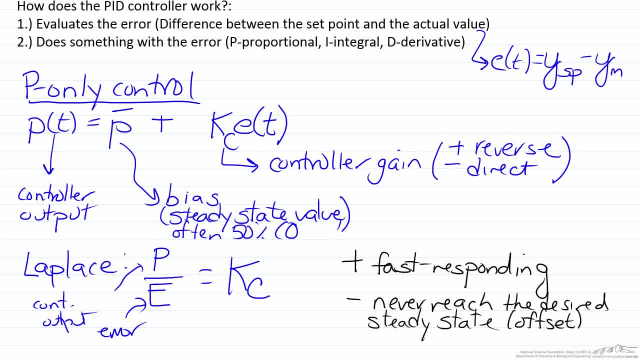 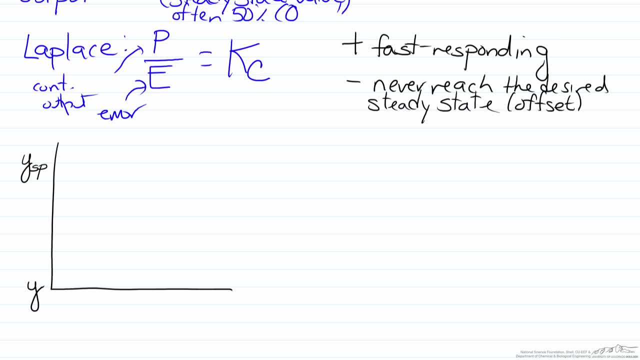 often referred to as the offset. So, for example, if we start at a place going from y and we increase the setpoint to a particular value, the goal would be to reach this new setpoint value. However, no matter what value of K sub C is the value of the setpoint, the value of the setpoint is the 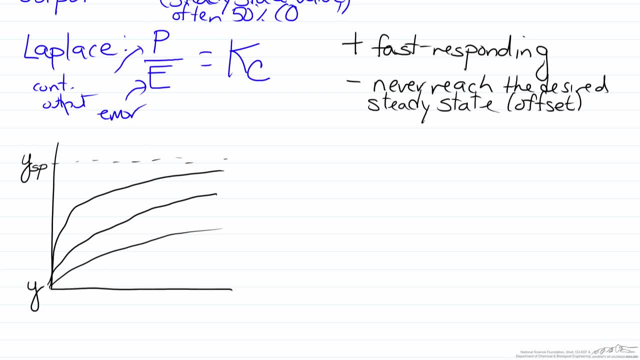 value of the setpoint If you select, the system will not reach its steady state. What we do know is that as K sub C is increased, the system will get closer to its steady state. However, as K sub C also goes up, the potential for stability issues also increases. So therefore, even though 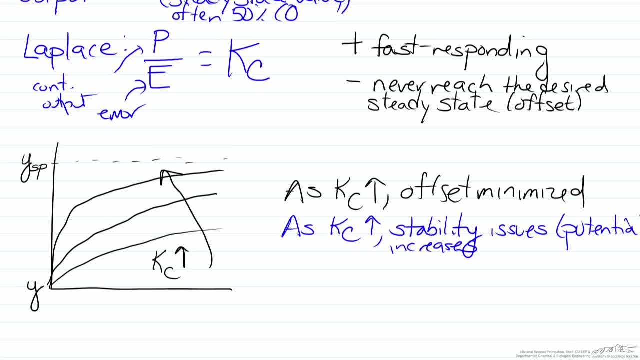 we've shown these responses as smooth over damped responses. it very well could be that your process could be introducing oscillations or potentially, in even a worse scenario, your process is now going to become unstable. So there is a trade-off here between the value of K sub C you select and in terms of the 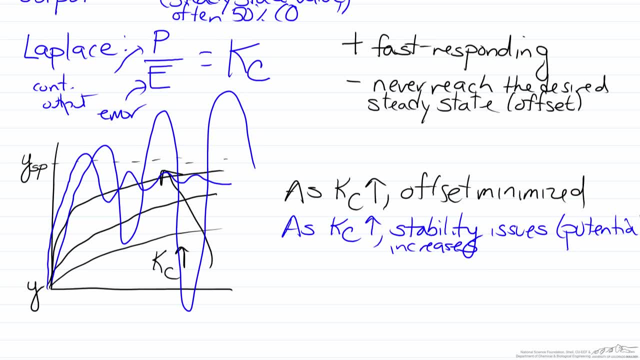 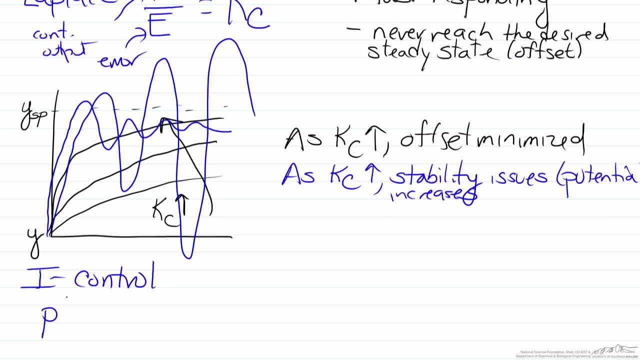 offset versus its issues for potentially being unstable. The next type of control is I control. As the name indicates, it handles the error by taking the integral of it. So here we'll have P of T equals P bar- again the bias plus. 1 over tau I multiplied by the integral of P bar. So we have P of T equals P bar times the bias plus 1 over tau I multiplied by the integral of P bar. So we'll have P of T equals P bar, again the bias plus 1 over tau I multiplied by the integral of P bar. So here we'll have P of T equals. 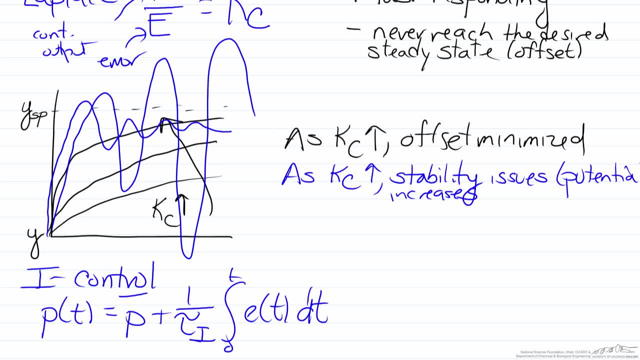 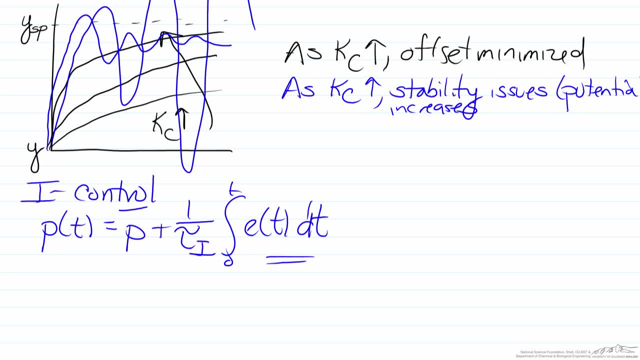 integral of zero to t of the error. By having this integral around, that will guarantee that our system will eventually reach zero error. How long it will take is another question in itself. This integral term eliminates offset And tau. i is known as the integral time or. 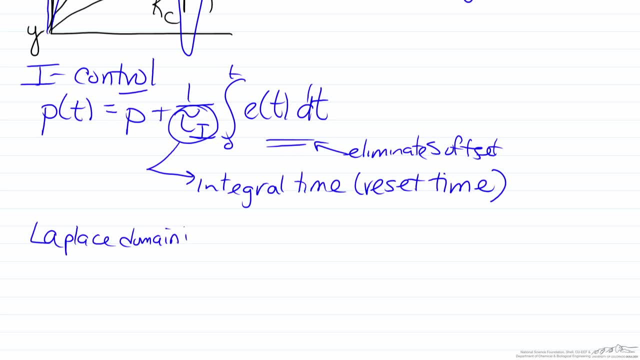 the reset time. In the Laplace domain, the transfer function p over e for an i only controller will be one over tau i s. So a good thing for i only control is that it eliminates offset. However, i control is very rarely used. There are a couple major reasons for this. The first: 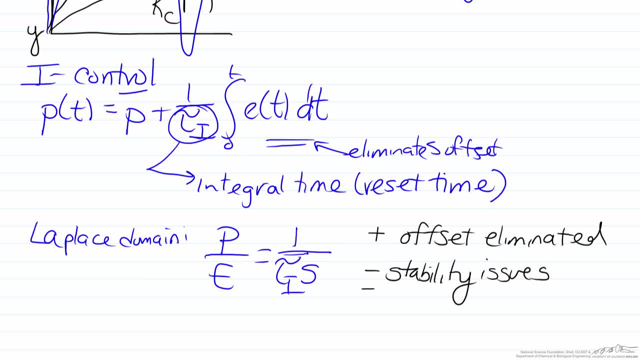 is that it is much more susceptible to stability issues. And secondly, the i control can't handle sustained error, because what will happen is that the controller will saturate, Because, even though error can go higher and higher and higher, a controller can only range. 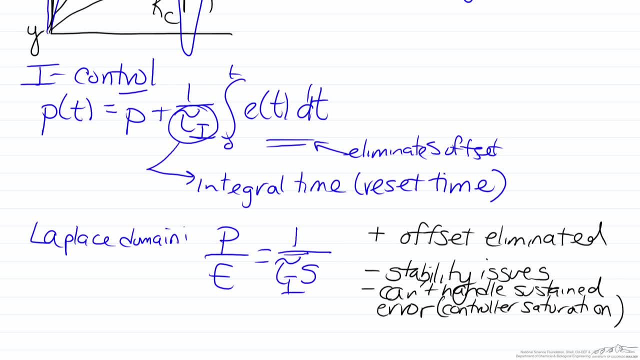 from zero to zero, From 0% controller output to 100% controller output. So therefore, often times, if the error is sustained and is of some large degree, the controller can't go beyond zero or beyond 100.. So therefore, it will get stuck there for a while, And what that means is that when 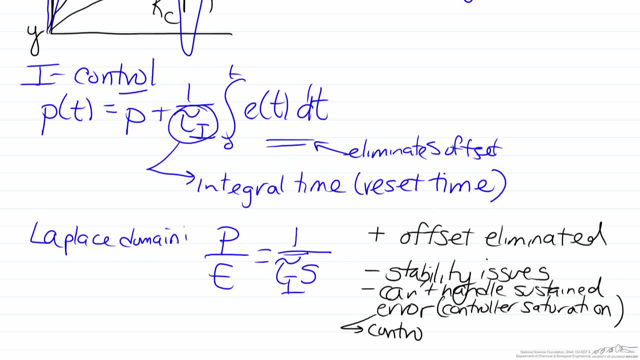 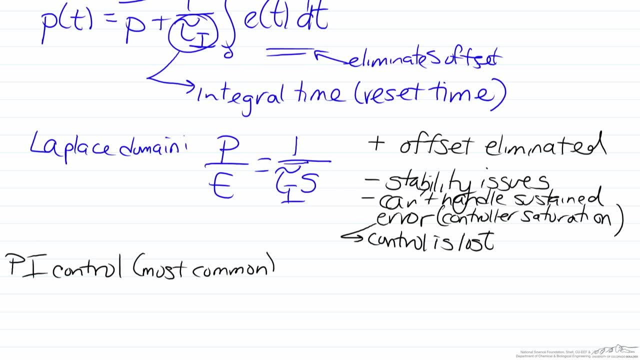 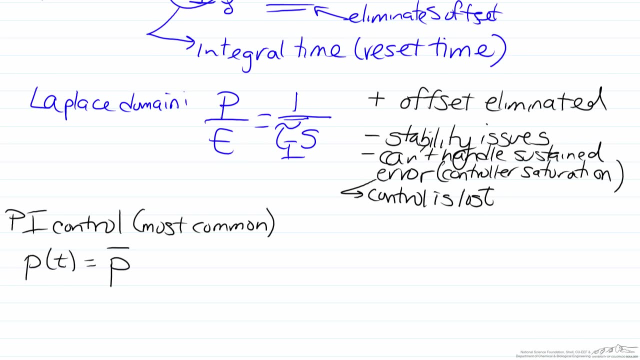 the controller, saturation happens. basically, control is lost. So therefore, p control is often used And p control, depending on your source, is recognized as the most common of the PID family, And what it literally represents is an addition of both the p part and the i part In the time domain and in the Laplace domain. 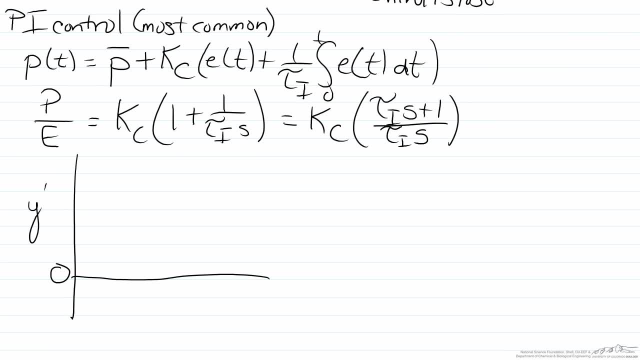 So here we'll look at a disturbance change. So therefore, when we see a disturbance change, what we would want to see is that the process returns back to the steady state, And if we're in deviation variables, that value would be zero. 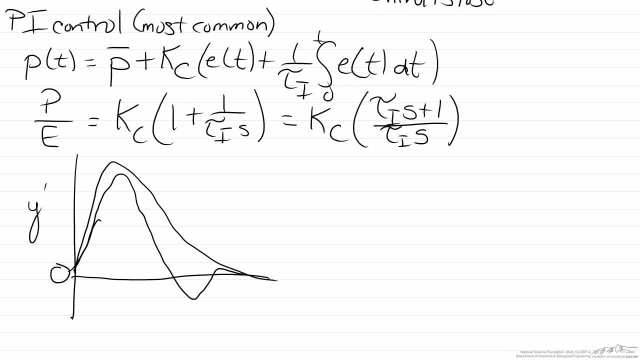 So the control system could look something like this: As tau i decreases, we see two things that happen. One is that the system reaches steady state much faster. Secondly is that the chance for stability issues rises. Again, these issues are similar to what we 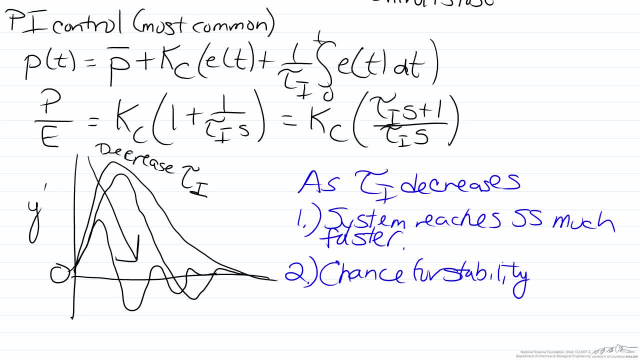 see for kc increasing, except instead of it reaching a steady state faster, although it does do that, the other issue is offset. So therefore, here the chance for stability issues increases, And you can see that here by the fact that you have more oscillations And 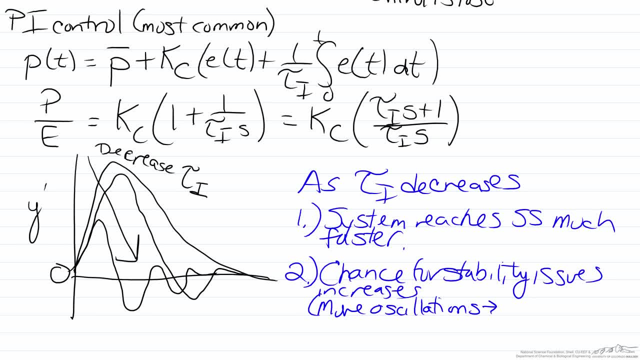 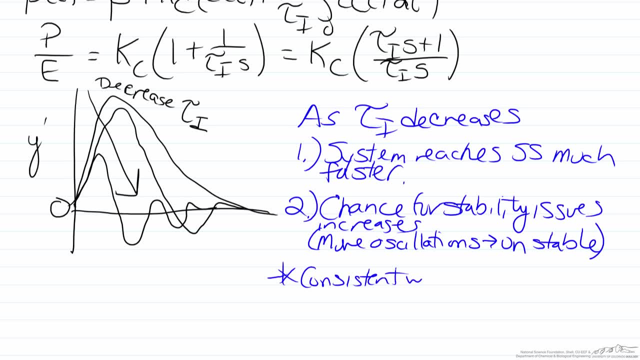 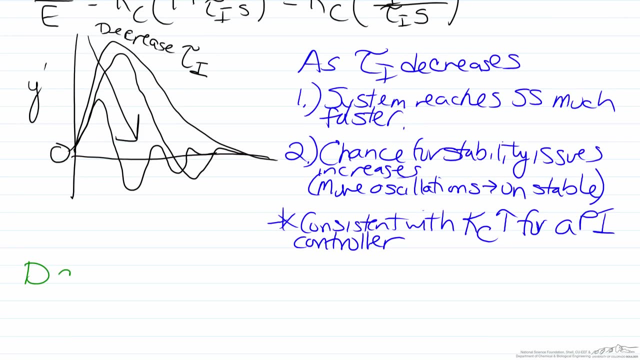 depending on your tuning parameters and your process. if you go too much higher, it can potentially go to an unstable process. These two effects are consistent with what happens as kc goes up for a PI controller. The final part of the PID family is D control. Remember that D stands for derivative, So 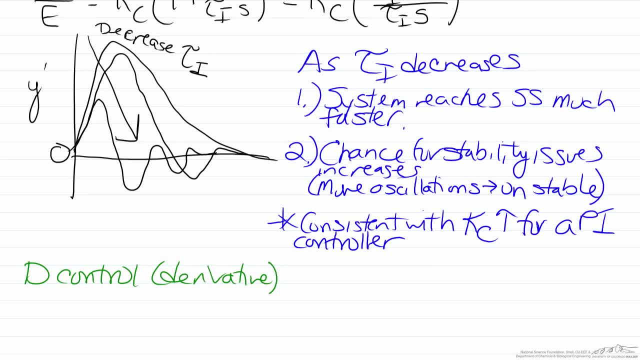 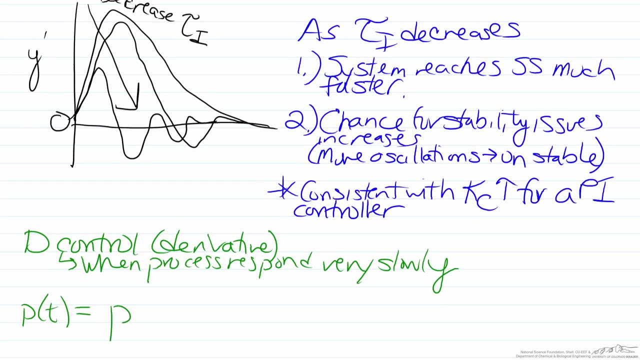 D control is not overwhelmingly used. It's really only particularly used for when processes respond very slowly. That is when D control comes in. And we can see why D control can help with this by looking at the equation. for D only control, It will be P, bar plus tau, D multiplied by the derivative. 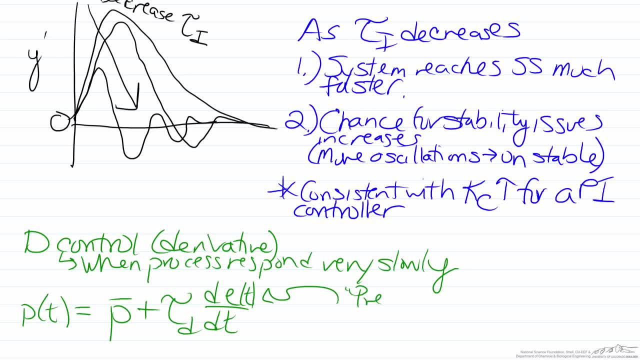 of the error. By using the derivative, it's acting as a predictive action, because by looking at how the slope of the error acts, you're predicting what direction your values are going to. So in the Laplace domain we can see this: We have P over E, which is the 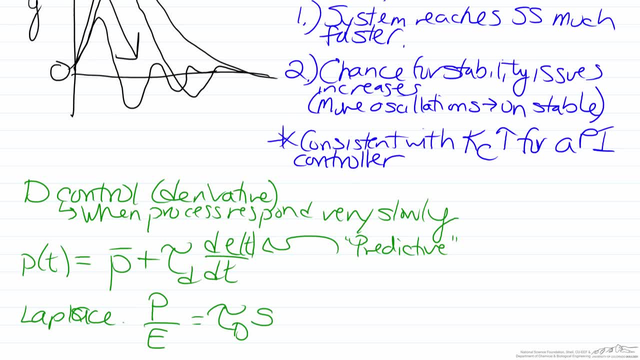 E equals tau D times S. So if you recall that when S is in the numerator of a process that means that it acts quicker, Whereas with S in the denominator it means it slows things down. The value of interest here is tau D, So tau D is known as the derivative time.